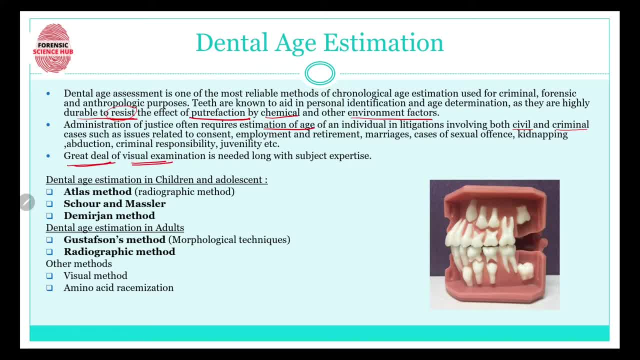 And for that we need a great deal of visual examination. Along with subject expertise. we need to be very much thorough with the knowledge. Other than the knowledge, we also need a great deal of visual examination. The forensic odontologist must thoroughly study each and every aspect of that particular teeth in order to determine the age of the person. 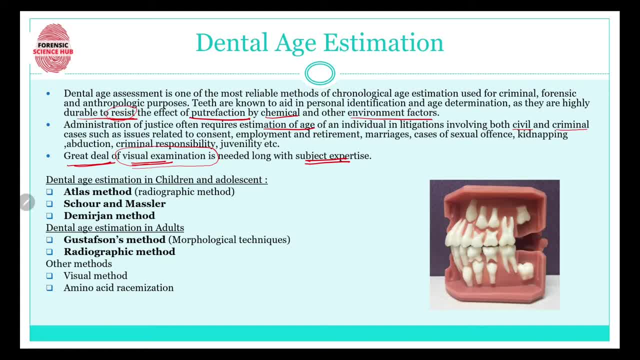 And hence visual examination is very important step in this. Now there are different methods for determining the age, So dental age estimation in child and in adolescent. There are three methods: that is atlas method, which is a radiographic method, Then there's Schur and Masler method. 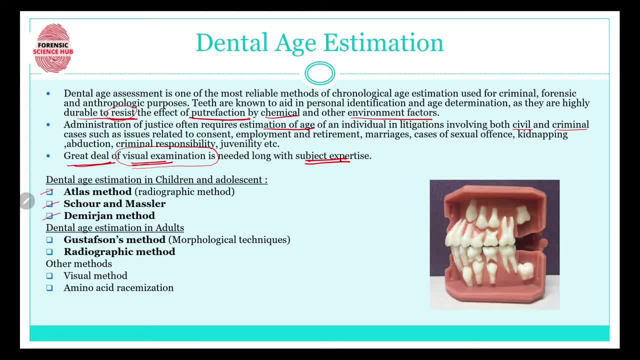 And then there's Demergen method. Then, for determining it in adults, we have Gustafsson radiological method, And there are some other methods like visual method, amino acid grismalization also. So in this video I'm going to be discussing about these three methods. 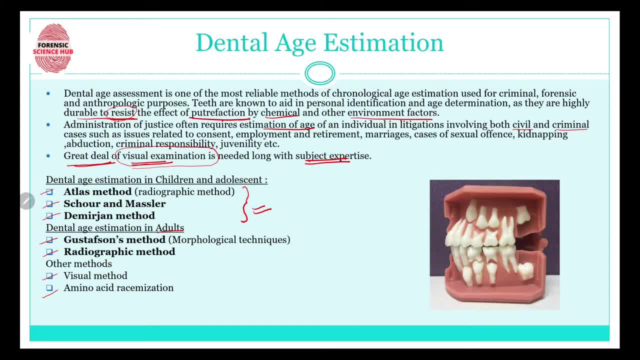 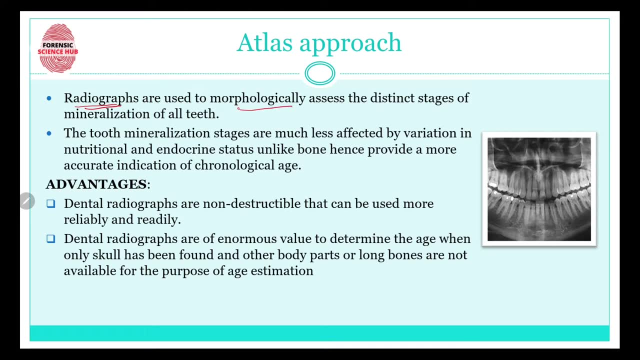 That is, the methods that are used for age estimation in children, And all the other methods will be discussed in my next video. So let's start with the atlas approach: Radiographs. In this method, radiographs are used to morphologically assess the distinct stages of mineralization of tooth. 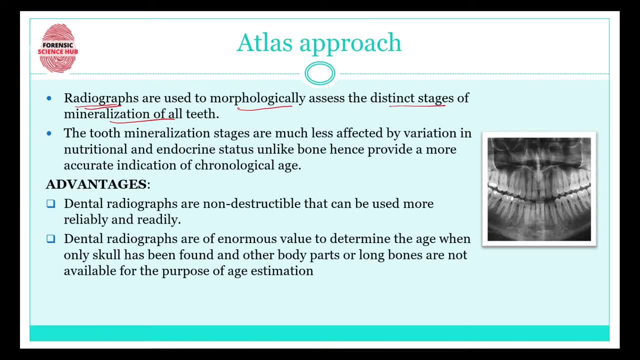 Radiograph is basically a static image that is generated when x-rays are passed through the tooth- In case teeth. So x-rays are used in this method and radiographs are made. This is a radiograph. This picture is a radiograph of teeth. 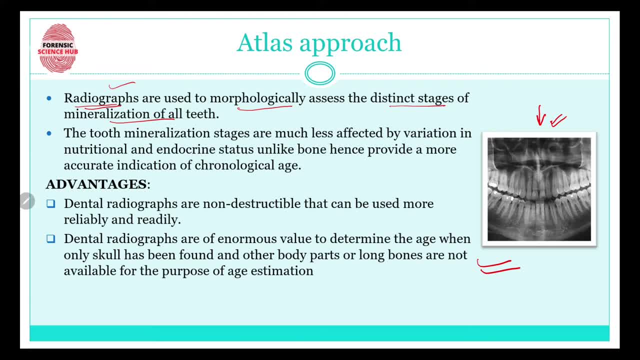 And with the help of these the odontologists are going to study the various stages. There are various stages of mineralization of teeth. So which stage the person's teeth were in We can determine that and on the basis of that, age of the person can be estimated. 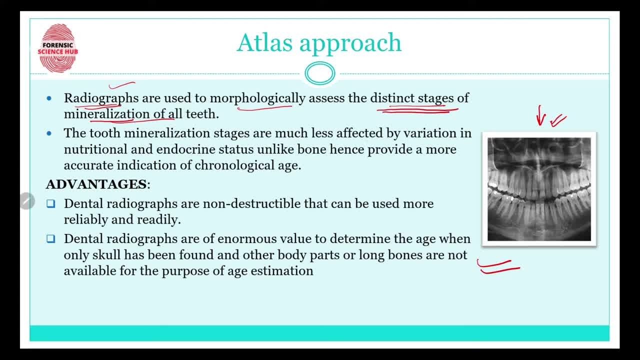 The tooth mineralization stages are much less affected by variation in nutritional and endocrine status, Unlike bones, hence provide a more accurate indication of chronological age. So any bone- in cases of bone bones are also mineralized. teeth are also mineralized, But the bones mineralization stages can be affected by the nutritional habits of the person or the endocrine status. 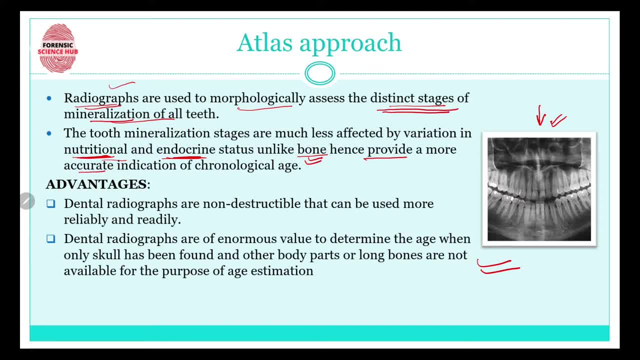 And hence it can. You know, we cannot determine the age. We cannot determine the age through that, But this is not so in teeths case. Teeth mineralization is not affected by this, by nutrition or by endocrine status. Hence it is more reliable. 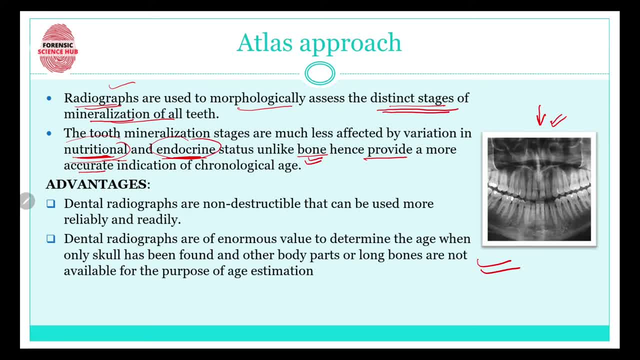 The advantages of atlas method is dental radiographs are non-destructible. Of course, these radiographs cannot be destructed. Also, the x-rays don't affect the teeth in any way, So dental radiographs can be used readily and reliably. Dental radiographs are of enormous value to determine the age, when only skull is found and other body parts or long bones are not available for the purpose of estimation. 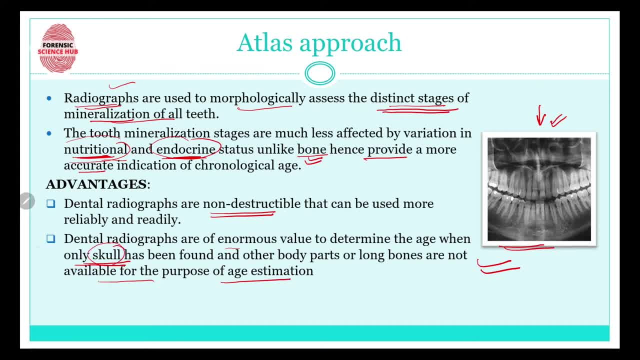 So when only skull is found, then dental radiographs become even more important, because we don't have any other part that we can look for age estimation. So in case of when only skull is present or available, then this becomes even more important. Then the second method is Shor and Masler's method. 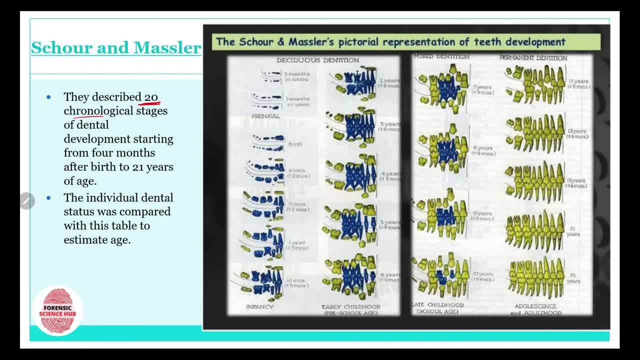 So Shor and Masler basically describe 20 different chronological stages of dental development, starting from 4 months age after birth to 21 years of age. Here is a picture that is showing all those 20 stages. The individual dental status was compared with this table to estimate age. 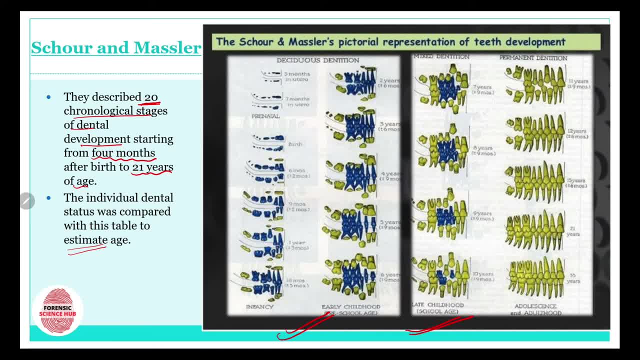 So here in this picture you can see Basically- this is a picture- The blue colored they are showing as the deciduous dentition of the primary teeth, Whereas this yellowish part is showing as the permanent teeth. First we have deciduous teeth. 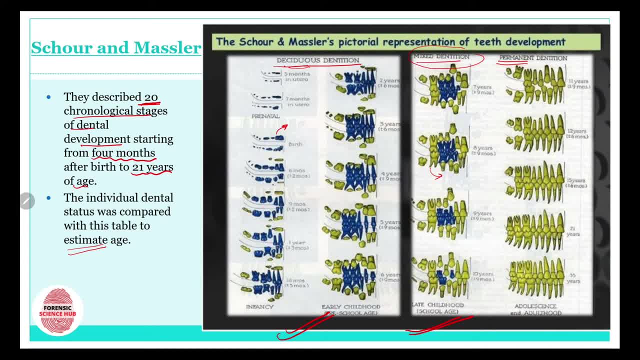 Then we have mixed dentition, That is, a mix of deciduous and permanent teeth. Then comes the finally permanent teeth. So in different stages, some of the teeth are erupting. Some are still inside the jaw, Like this is inside the jaw. 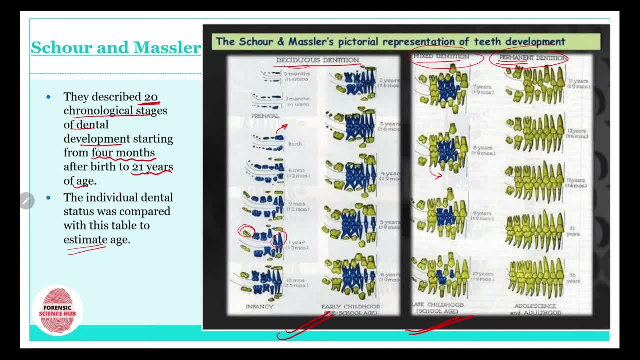 These are erupting. So there are various stages And if we have a set of teeth, we need to estimate the person's age. Then what we can do is we can study those teeth. We can see how many have erupted, how many are still inside. 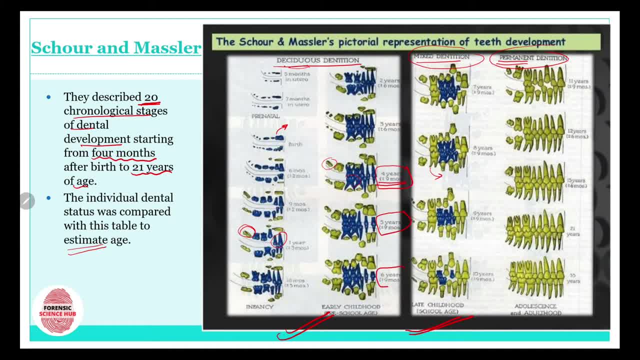 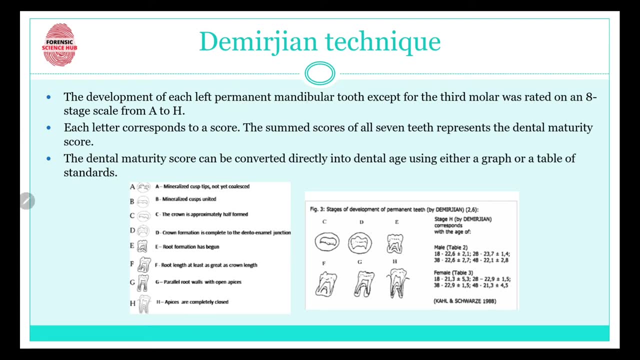 And on the basis of that we have the estimated age written over here in this chart, So the individual dental status can be compared with this table to estimate the age. Then we have Demirjan's technique. The development of each permanent mandibular tooth, except for the third molar, was rated on eight stages, from A to H. 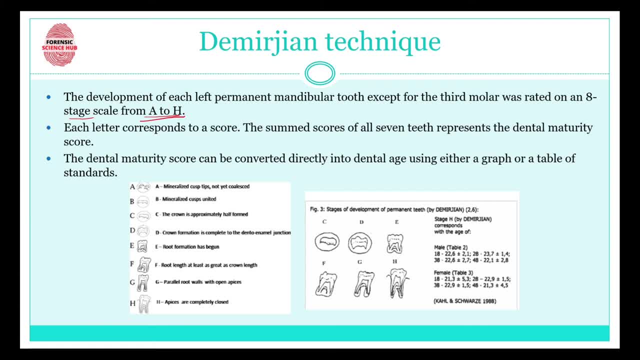 So, basically, Demirjan, he rated the teeth on eight scales that started from A to H, A, B, C, D, E, F, G and H. Each letter corresponds to a score. The sum score of all the seven teeth represents the dental maturity score. 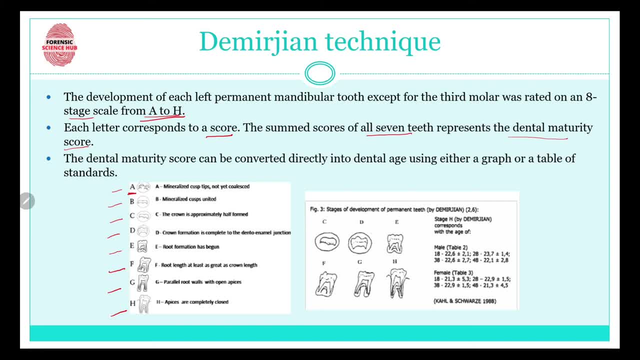 And these scales mean different stages, Like for example: A here means mineralized cusps, tips not yet coalesced. B means mineral cusps united. C means the crown is approximately half formed. D means crown formation is complete to dental enamel junction. 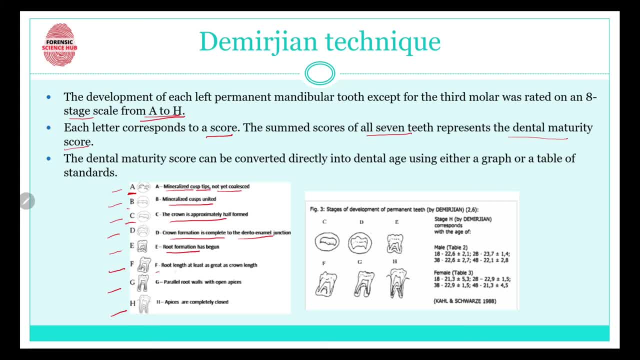 E means root formation has become. F means root length at least as great as crown length. G means parallel root walls with open apices. H means root length at least as great as crown length. H means apices are completely closed. So these are various stages that are given. 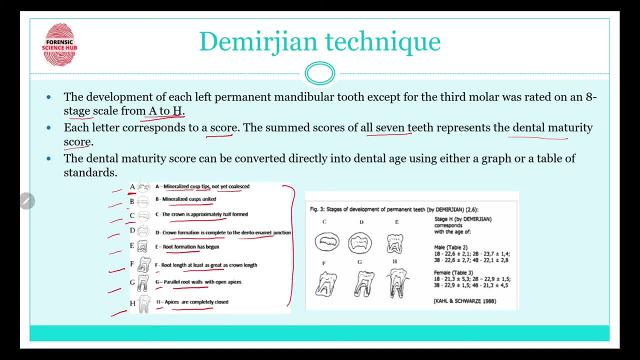 So we have this, Then we have the teeth that we have to estimate the age of. We are going to sum the scores of all the seven teeths And then we are going to get a dental maturity score. The dental maturity score can be converted directly into dental age by using a graph or a table of standards. 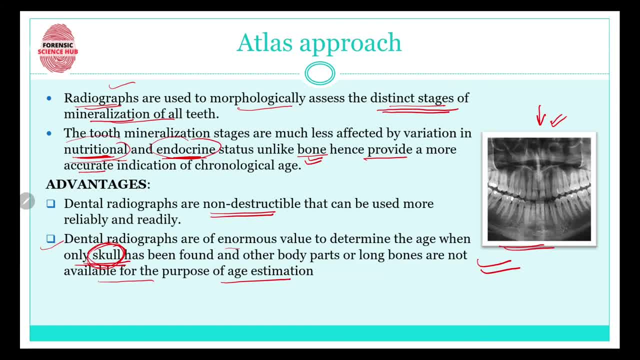 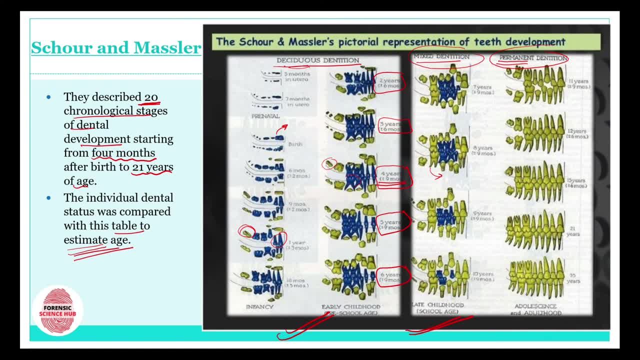 So I hope you understood these three techniques. Atlas approach used radiographs And then the mineralization stages were studied: Ensure and Vassler. There were 20 chronological stages that were representing the teeth development Which can be used to compare the individual dental status of a person. 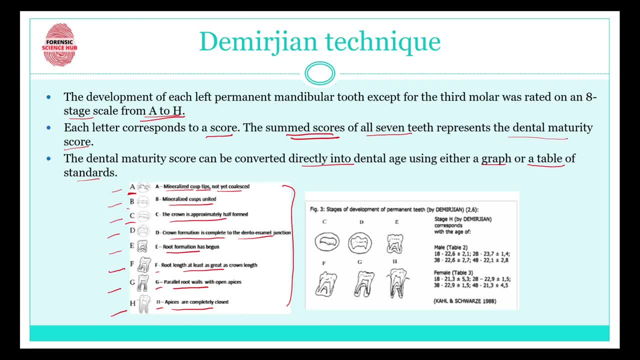 Then Demirjan's technique rated different teeths from A to H, And then those scores were summed And the dental maturity score was converted then into dental age. So this was all about this video. Thank you for watching.